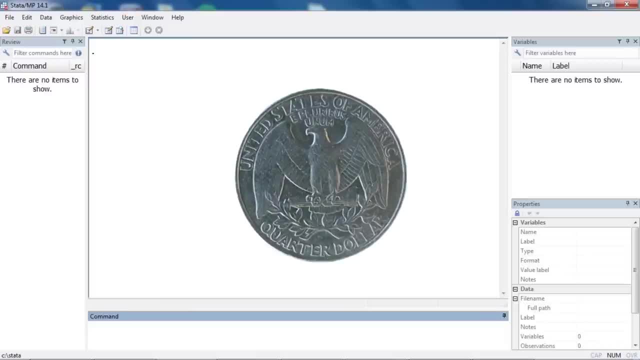 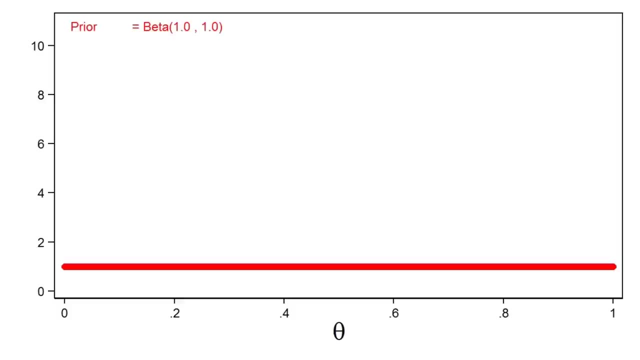 This side is often called the head side and the other side is called the tail side. If I toss the coin in the air, it must land on either the head side or the tail side, and we could use theta to denote the probability that the coin lands with the head side facing. 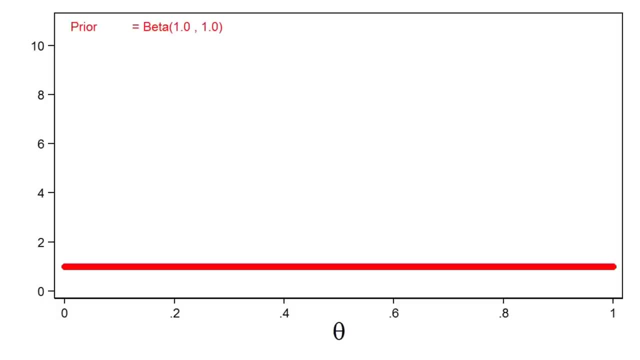 up. Since I don't have any data, I could use a uniform distribution to express the belief that the probability of heads could be anywhere between 0 and 1 with equal probability. Here I've used a beta distribution with parameters 1 and 1, which is equivalent to a uniform distribution on the interval 0 to 1.. 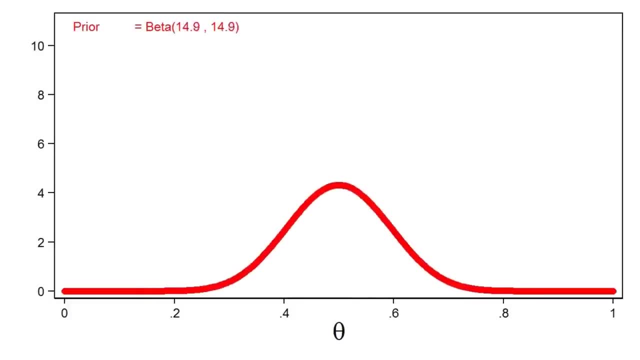 But common sense would suggest that the probability of heads is closer to 0.5, and we could express this belief mathematically by increasing the parameters of our beta distribution, which would concentrate the probability closer to 0.5.. This mathematical expression of our belief. 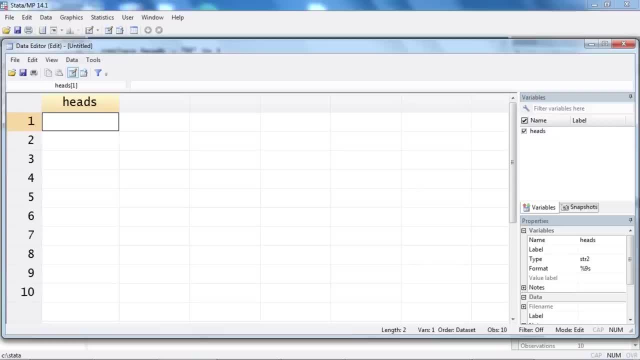 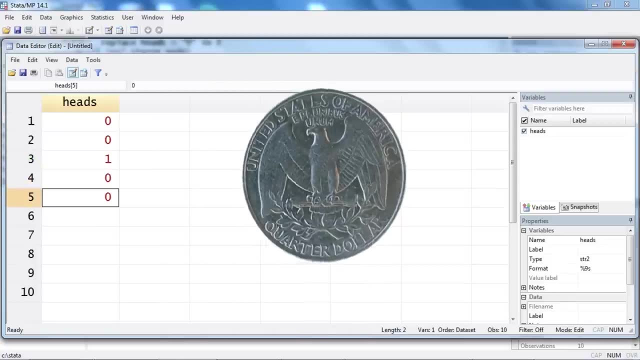 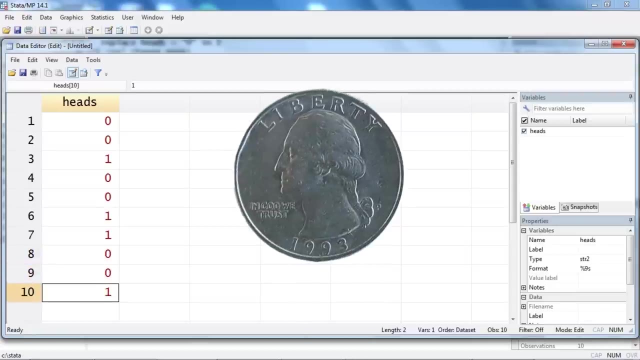 about. the parameter is called the prior distribution. We could also investigate the value of theta by conducting an experiment. We could flip the coin 10 times and calculate the proportion of times that the coin lands with the head side up. Here we observe 4 heads out of 10 tosses of the coin. 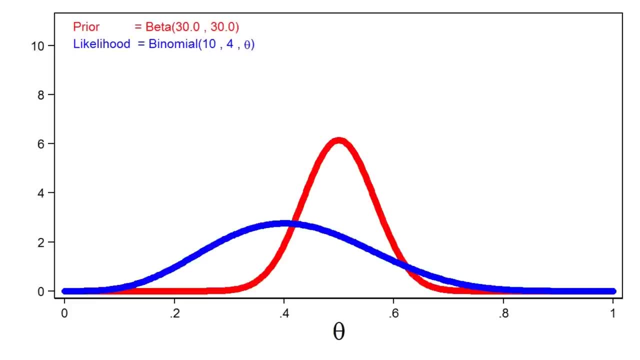 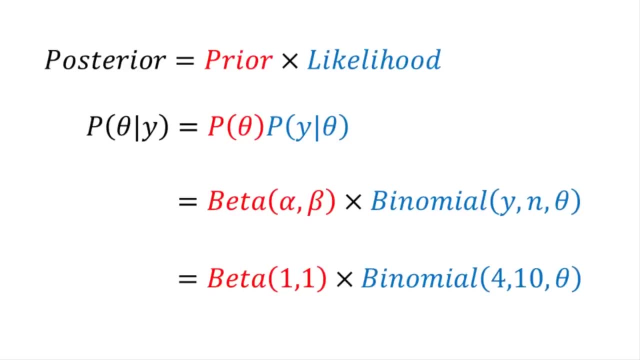 We can quantify the results of our experiment using a likelihood function. In this case, the blue line displays a binomial likelihood function for theta, given 4 heads out of 10 coin tosses, Bayesian analysis allows us to update our belief about the parameter with the results. 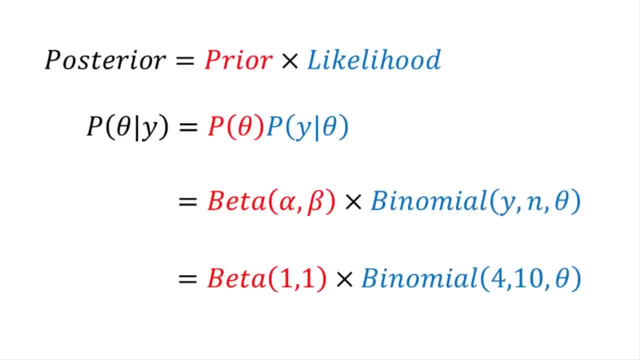 of our experiment. In simple cases we can compute a posterior distribution for the parameter by multiplying the prior distribution and the likelihood function. In this example, the beta distribution is called a conjugate prior for the binomial likelihood function because the posterior distribution belongs to the same distribution family as the prior. 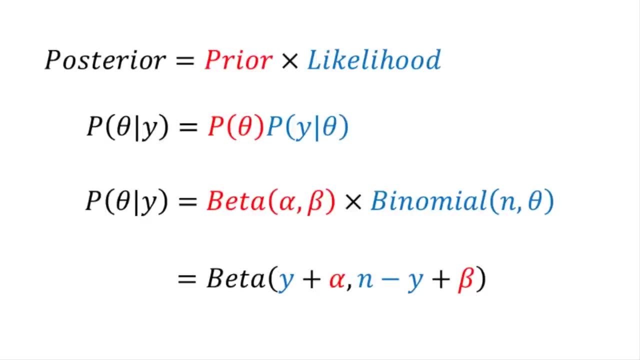 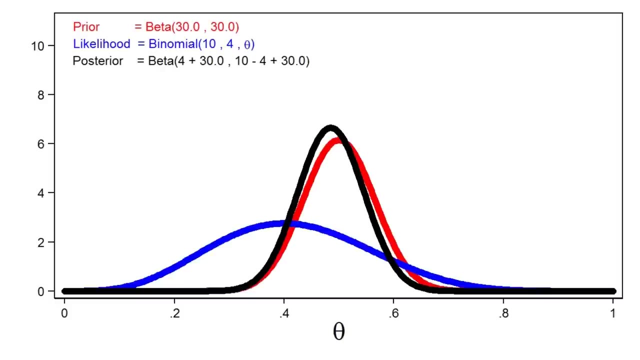 distribution. Both the prior and the posterior have beta distributions. Here I've plotted the posterior distribution of theta with the prior distribution and the likelihood function. Notice that the posterior closely resembles the prior distribution. This is because we used an informative prior and a relatively small sample size. 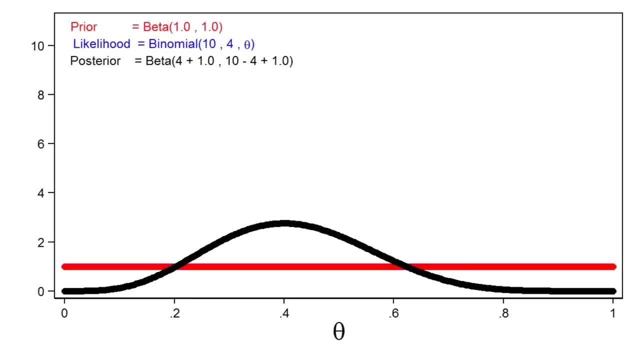 Let's look at the effect of different priors on the posterior distribution. Here the red line represents a completely uninformative prior in the form of a beta distribution with parameters 1 and 1.. The likelihood function is plotted in blue, but it is masked by the 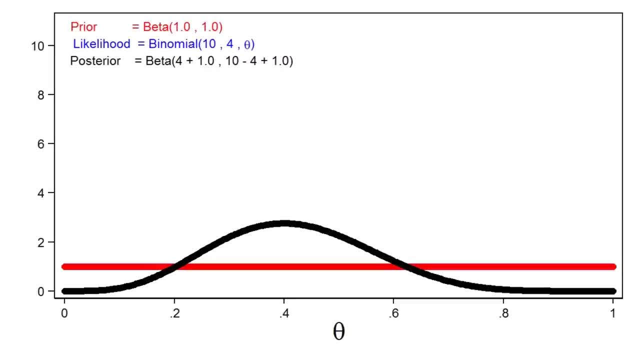 posterior distribution, which is plotted in black. This is an important feature of Bayesian analysis. The posterior distribution will usually be equivalent to the likelihood function when we use completely uninformative priors. The animation shows that more informative priors will have greater influence on the. 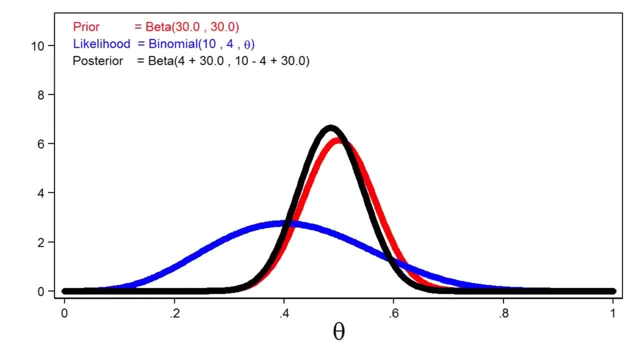 posterior distribution for a given sample size, And this animation shows that larger sample sizes will give the likelihood function more influence on the posterior distribution for a given prior distribution. In practice, this means that we can obtain precise estimates of the posterior distribution using smaller sample sizes when we use more. 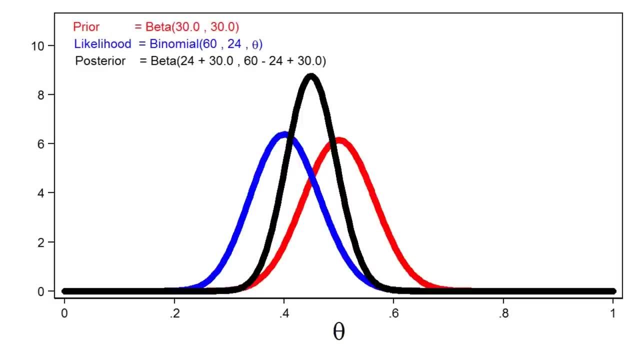 informative priors, But similar precision may require a larger sample size when we use a weak or uninformative prior. We can use the posterior distribution to calculate various quantities. For example, we can calculate the mean of the posterior distribution or the median or the mode, if we wanted and we 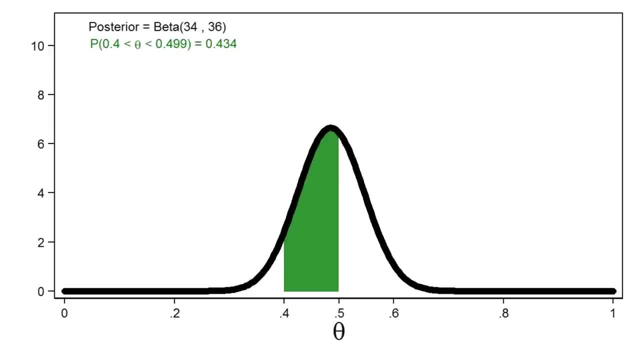 can calculate the probability that theta lies within an interval such as 0.4 to 0.5.. And similarly, we can calculate a 95 percent equal tail credible interval. We can also calculate a highest posterior density credible interval, also known as. 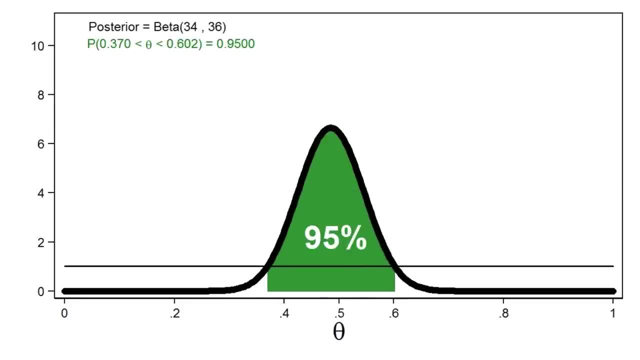 an HPD credible interval. The calculation of the HPD credible intervals is often described as dropping a horizontal line through the density until the probability within the interval equals 95 percent or 0.95.. For a symmetric distribution, the equal tail and the HPD 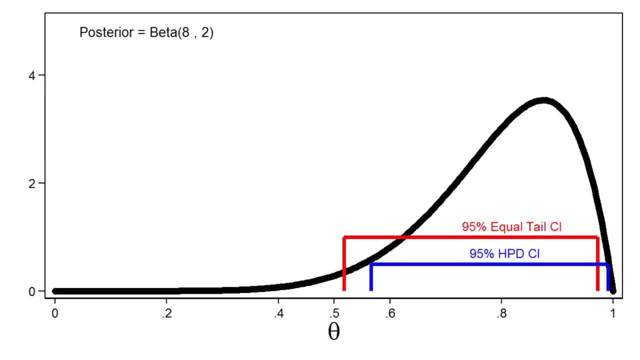 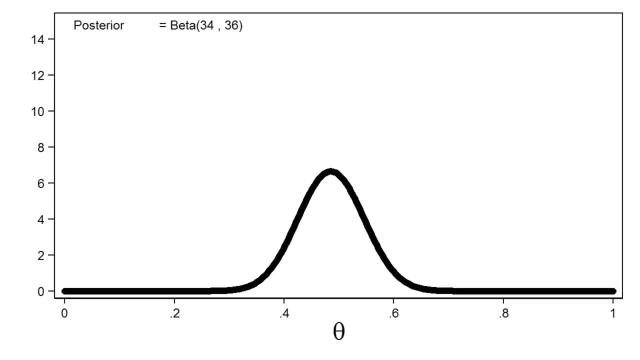 credible intervals will look very similar, but they will look very different for skewed distributions. One nice feature of the Bayesian approach to statistics is that the posterior distribution from a previous study can often serve as the prior distribution for subsequent studies. Here we've used the posterior distribution as the prior for an experiment with a sample size of 100. 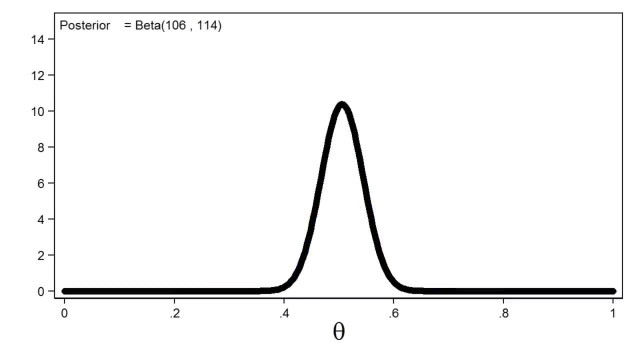 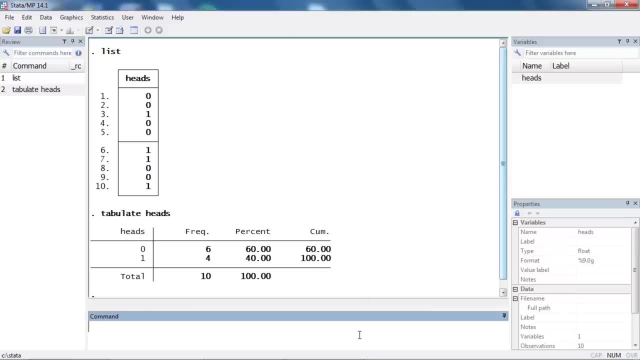 The resulting posterior from this experiment has an even narrower distribution, and we can then calculate the posterior mean and 95% credible interval for theta. So how do we do this in Stata? Well, here I've simply typed in the raw data: zero represents tails, one represents heads, and at the bottom I've tabulated the variable heads. 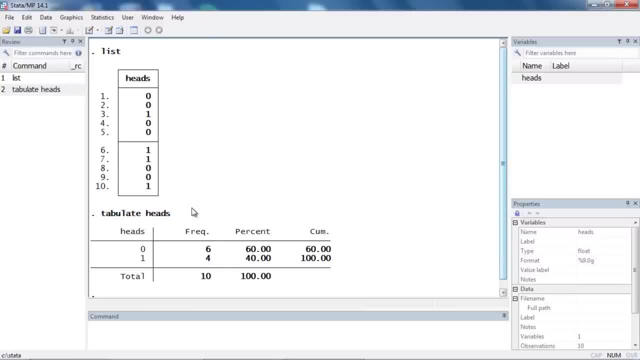 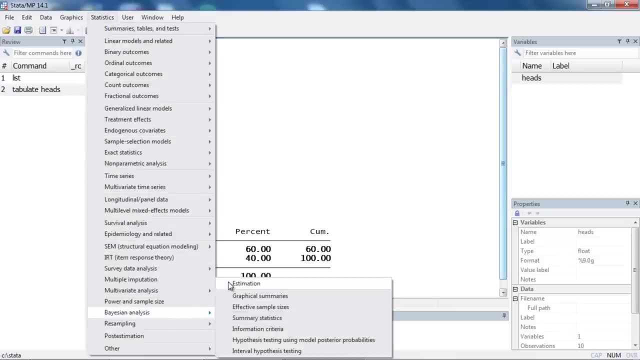 and I can see that there are six tails and four heads. So if I wanted to fit a Bayesian model, I can go to statistics and then scroll down to Bayesian analysis and then select estimation, and then this will open the Bayes-MH dialog box. So the first thing we need to do in the model tab, 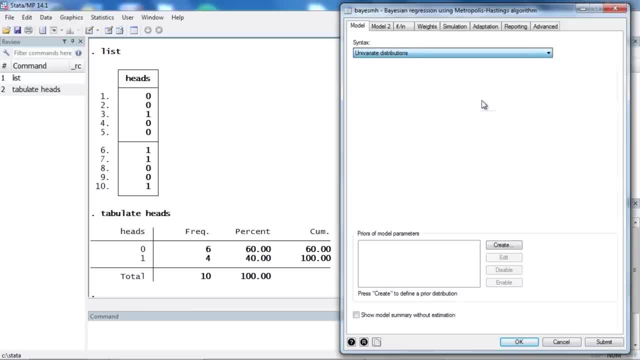 under syntax is we need to select univariate distributions and then, under model, we need to select a dependent variable, which in this case is heads. There are no independent variables in this case. Next, we need to specify a likelihood, function or distribution, as well as our priors. So for 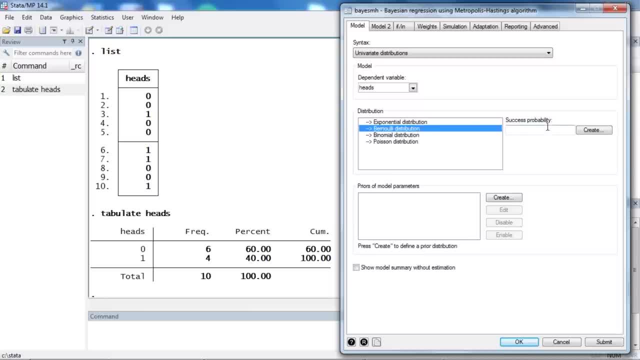 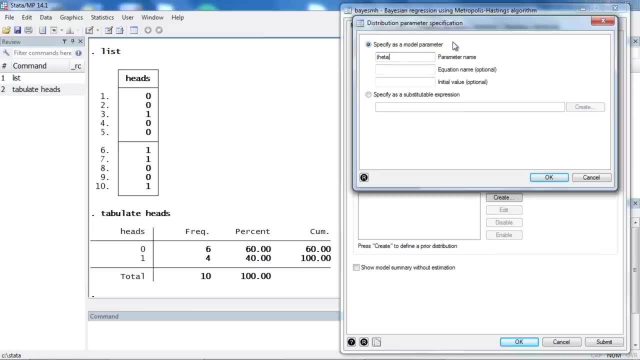 the distribution. I'm going to select Bernoulli distribution and then for the success probability, I'm going to click create and I need to specify a parameter name. So I'm going to call my parameter name theta. and there's some other options here, but we'll come back and talk about those in other. 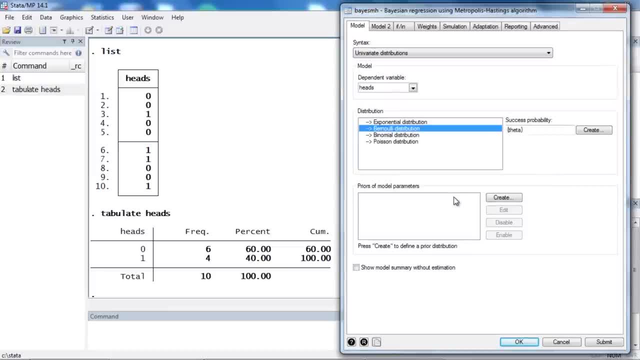 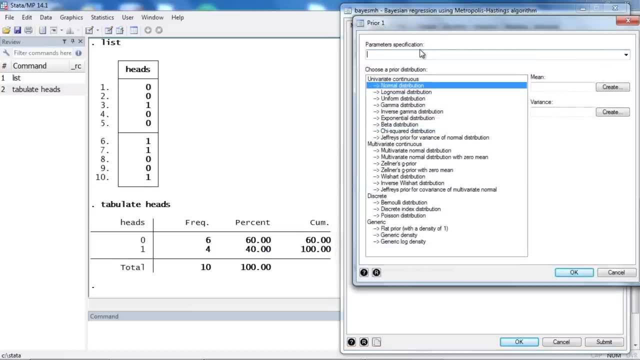 videos. For now, I just need a name for my parameter. Then the next thing I need to do is select the priors for my parameter or prior. So let's click create and then, at the top of the prior dialog box, I need to select which parameter, which in this case is theta. it's the only one. 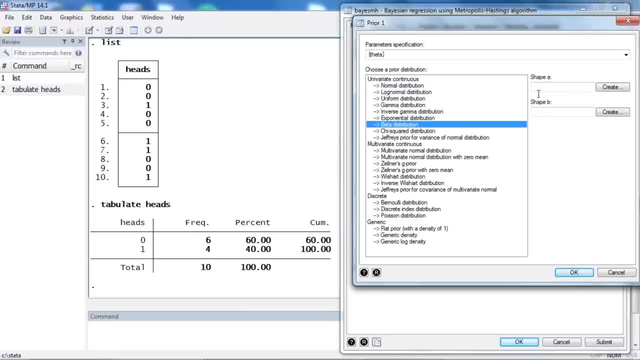 and then I need to choose a prior distribution. In this case, I'm going to use a beta distribution, and for shape parameter a, I'm going to use one, and shape parameter b, I'm going to use one as well. This is a the beta version of a uniform distribution. Then I'm going to click OK. 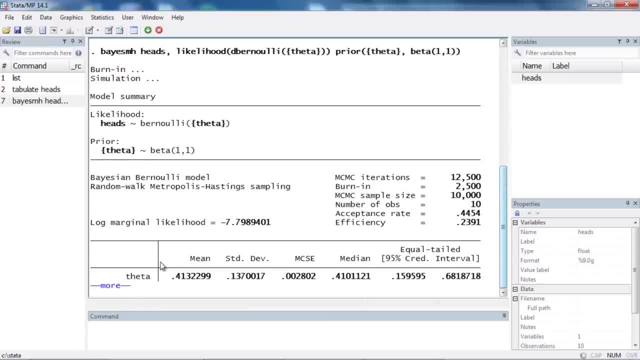 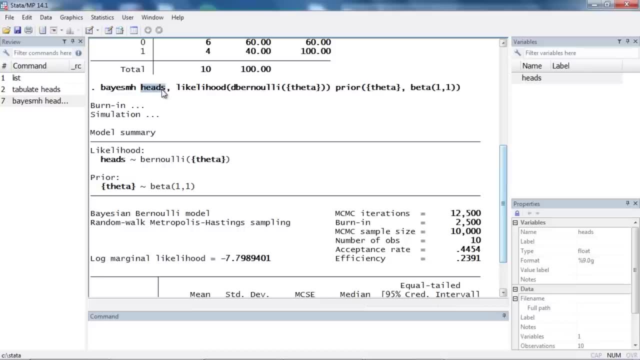 and then click submit. And in the results window let's take a look at the command. here The command is base mh, followed by the dependent variable heads, and then I can see my likelihood function specified as theta, Bernoulli likelihood with parameter theta, and then I have a prior for the 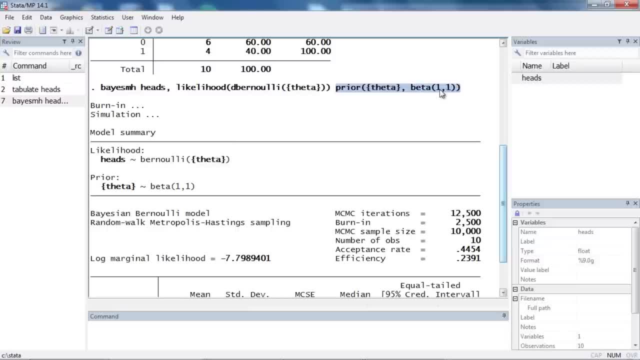 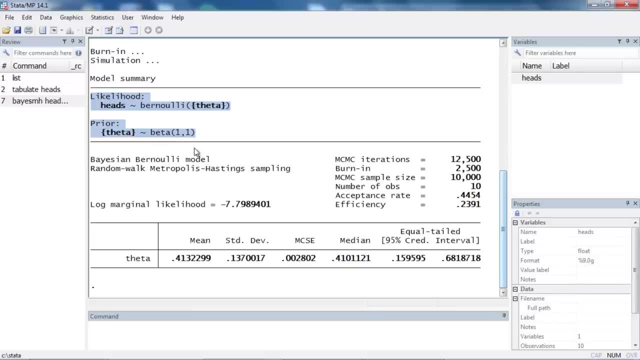 parameter theta, in which case, in this case, the prior is a beta 1: 1 distribution. Then if I look further down in my output, I can see that the command echoes the likelihood in the prior. It also shows me some information about the uh, the MCMC iterations and so forth, and we're going to come back and talk about that in the 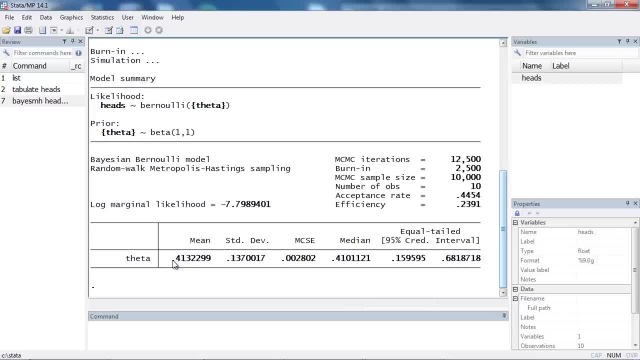 next video. So let's just skip to the bottom. here We can see that the mean for theta is 0.4132.. The standard deviation is 0.1370 for theta. Then we have our MCSC, our Monte Carlo standard error.